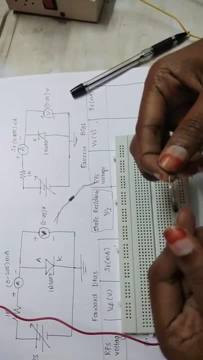 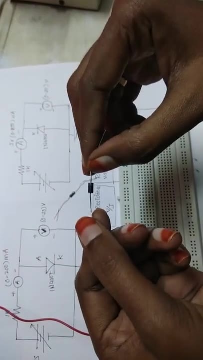 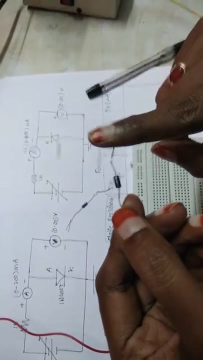 So let us do the reverse bias characteristics of the PN diode. Already we know that. so this is anode, the silver coated line set is cathode. So reverse bias, in the sense the positive terminal of the RPS is connected to the cathode and negative terminal of the RPS is connected to the anode. 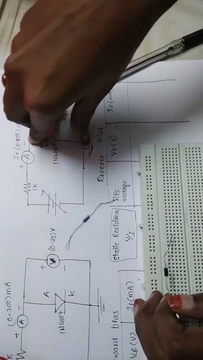 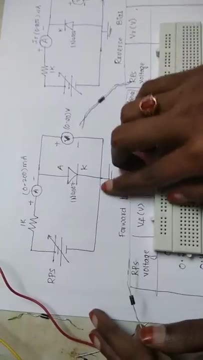 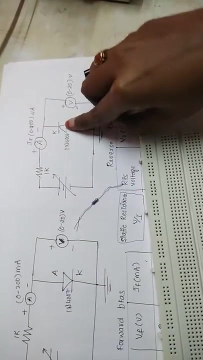 So once you observe this diagram, I simply changing the diode direction instead of changing the supply. So can you see the difference between forward and reverse? So for forward, just, I am connecting positive to anode, negative to cathode. For reverse, I am changing the directions of the diode: Cathode is connected to positive, anode is connected to drop. 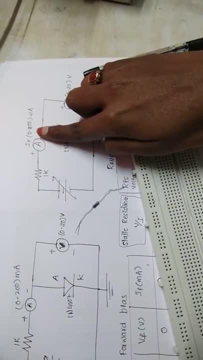 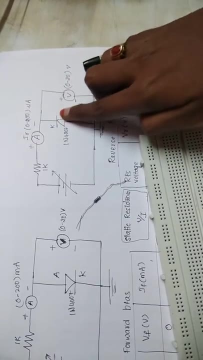 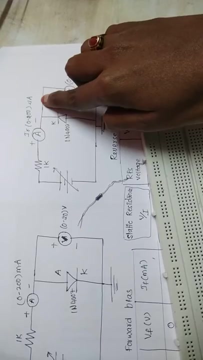 So, but here I am using 0 to 200 microampere, some meter. Why? Because here I am connecting diode in reverse bias, So the current, the reverse current, is very less in silicon diode, So it is in microamperes, So the reverse current is less. That's why I am using microamperes some meter. So let us build a circuit. 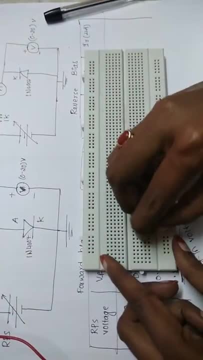 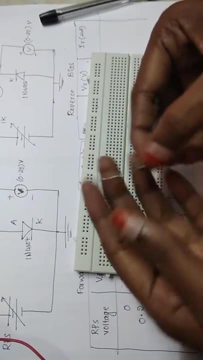 So first I am connecting the 1 kilo ohm resistor. So here I am connecting 1 kilo ohm resistor. Next I am connecting the diode. So here reverse bias, in the sense anode is connected to the anode. 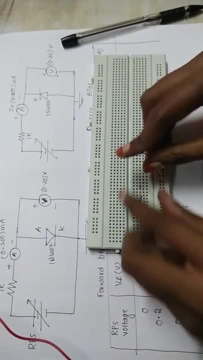 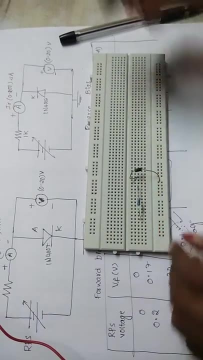 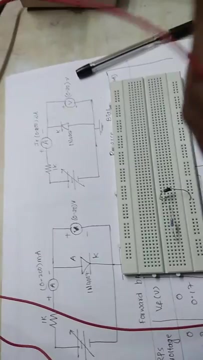 From the ground I am taking. this one is ground, this one is VCC. So, just simply, I am connecting two components. Next, I am connecting RPS. RPS positive is connected to the first end of the resistor, So rps positive is connected to the first. 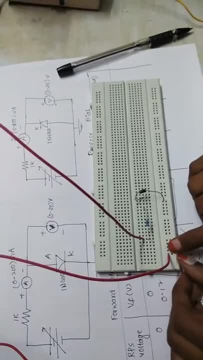 end of the resistor. rps negative is connected to the ground. These are in same horizontal Herzegovina, these are in same vertical websites. So what needs to be done is to connect these two components So You take that one foritter around the ground. 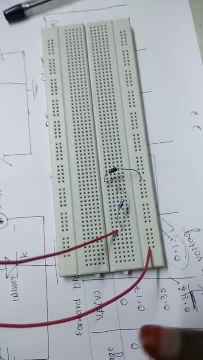 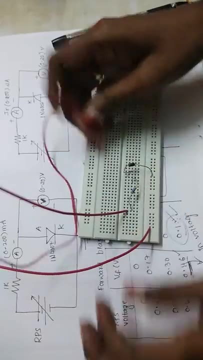 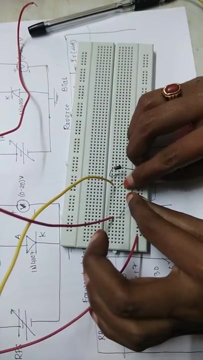 are in same vertical line. These are in same horizontal line. Next, I am connecting the ammeter. So here I am using the micro amperes ammeter. So ammeter positive is connected to the second end of the resistor, Same vertical line, And ammeter negative is connected to.